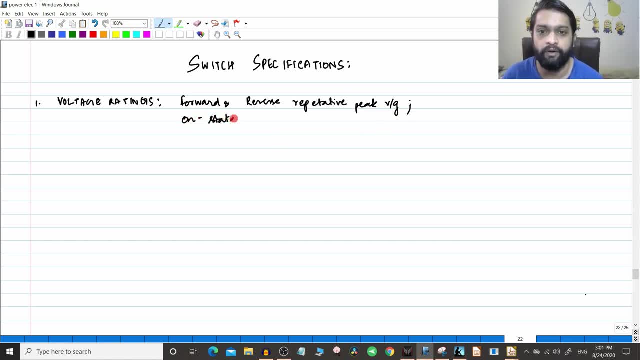 give something which is called the on state forward voltage drop. We have already seen this side on state forward voltage drop And, in ideal case, we have told you that this on state forward voltage drop should be tending to 0 and the forward and reverse repetitive. 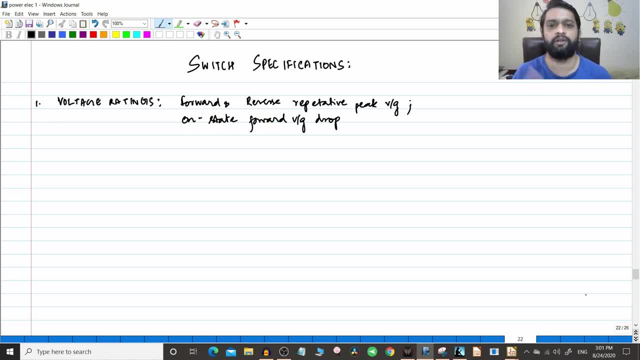 peak voltage, that is, forward voltage, is what voltage? forward voltage is the voltage which is you are applying on the SCR and the reverse voltage is also which you are applying on the SCR. So they are talking about the peak voltage, not the RMS voltage. they are talking 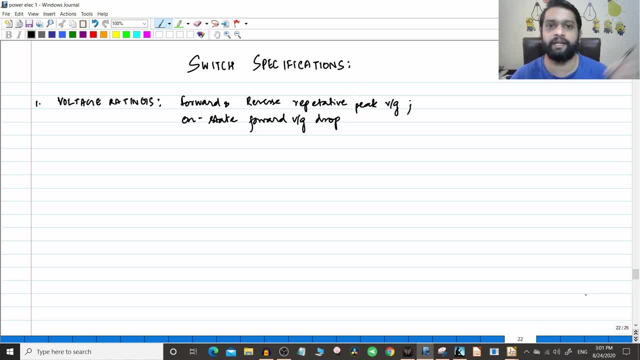 about the peak voltage case of AC signal etc. you are going to have an alternating wave, So they are talking about the peak voltage. Next one is the current ratings. So current ratings, you can have the average current ratings. you can have average current ratings. 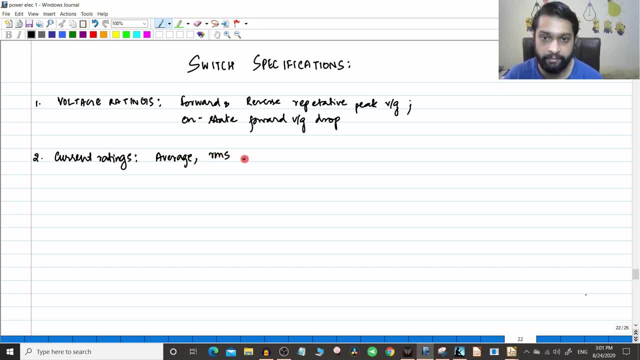 ratings: okay, you can have the rms- current ratings. okay. then you can have the repetitive peak. okay, and then you can have also something which is called the non-repetitive peak. non-repetitive peak- these are all self-explanatory. and then you can have the off state leakage. 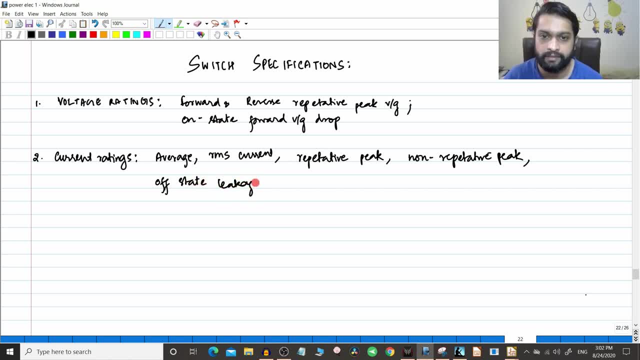 current. off state leakage current. okay, so these are basically the ratings of the switch. that means how much average rms current average current it can take, how much rms current it can take, then the peak voltages for repetitive case and the non-repetitive. these are not that. 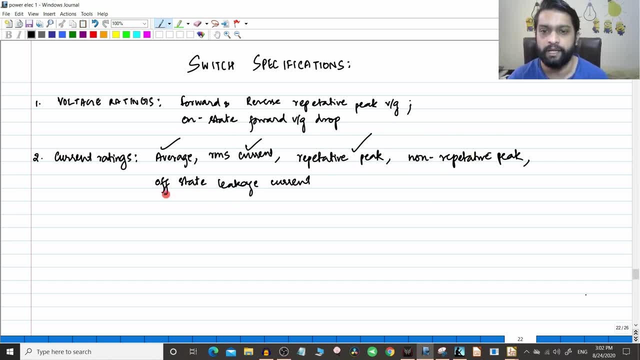 important. at this point of time, when we see the devices, we will see all these things much more. and then, of course, off state leakage current. now, off state leakage current, i told you for ideal switch it should be tending to zero, okay, and then average rms also. these things should be ideally. 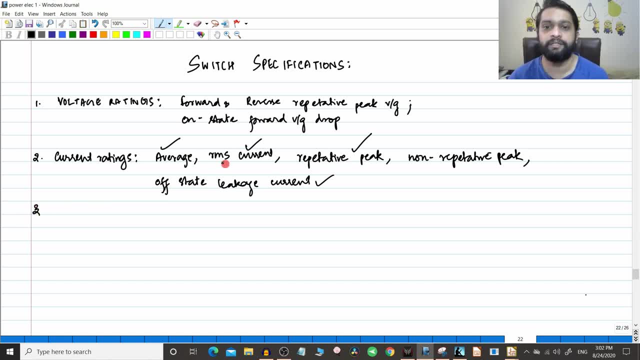 tending to infinity. okay, but in practical switches you don't have that infinite condition, so the manufacturer will give all these voltage so that you can design your system accordingly, okay, next is the switching speed: switching speed or frequency, switching speed or switching frequency. so this also, ideally, should be allowed. very high switching frequency should be there, right? so, of course, 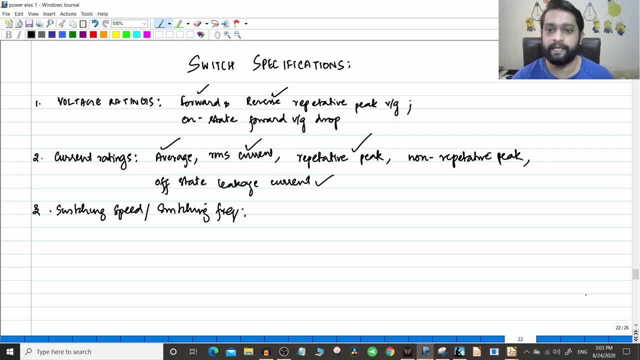 nowadays, there are devices which are having a very high switching speed. there are, specifically, devices which can handle such types of high switching speed. one kilohertz, one megahertz, all those things. okay, now this switching frequency, fs, is equal to 1 by ts, which is 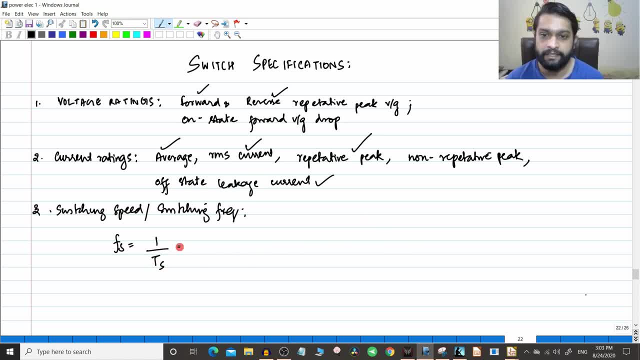 called the switching time period. we have seen that in the previous video and the switching time period was what the switching time period is: nothing but the delay time plus rise time, plus the normal operation time, plus the storage time, plus the fault time plus the off time. okay, off time. this is not turn off time, this is off time. turn off time is. 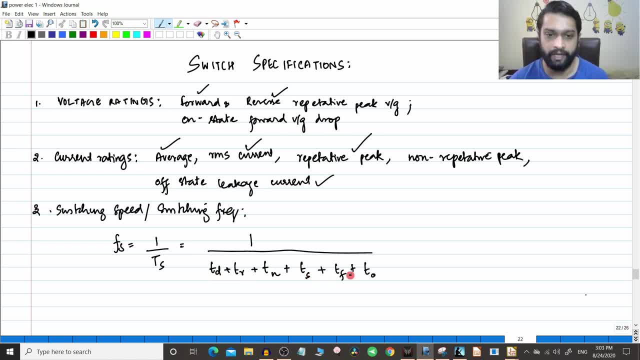 s plus t f, then the turn on time is t d plus t r. okay, so this is the switching frequency. so t 0 is called the off time of time. so, for example, in the textbook, what they have done, they have taken all these values, that is, t d is equal to t, r is equal to t, n is equal to t, s is equal to t, f is. 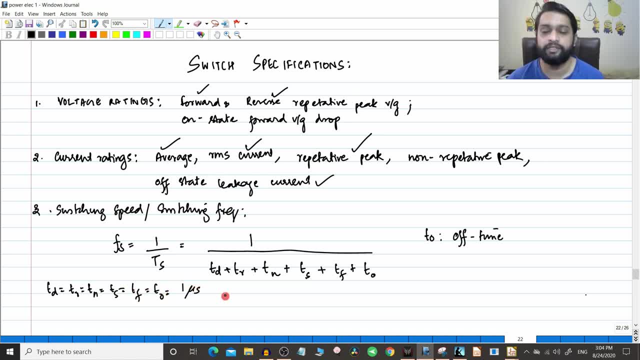 equal to t 0 to be 1 microsecond. okay, so the ts value will be 6 microseconds. so if you calculate like this, fs will be equal to 1 by 6 microseconds and it is 166.67 kilohertz. it means your switching. 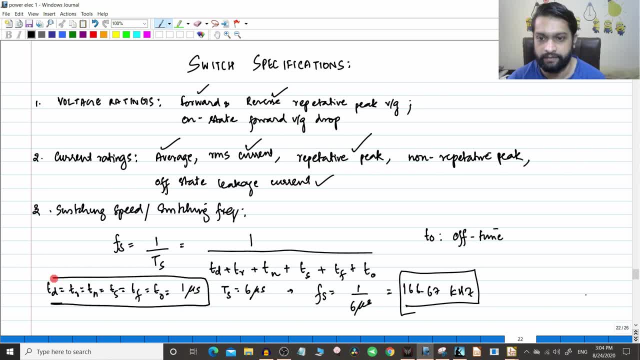 frequency limit, for example. the manufacturer gives all these values. okay, so your switching frequency limit will be 166.67 kilo. you cannot have pulses coming faster than this rate, so all your pulses, or your circuit, should be designed to handle pulses or give pulses less than this value. 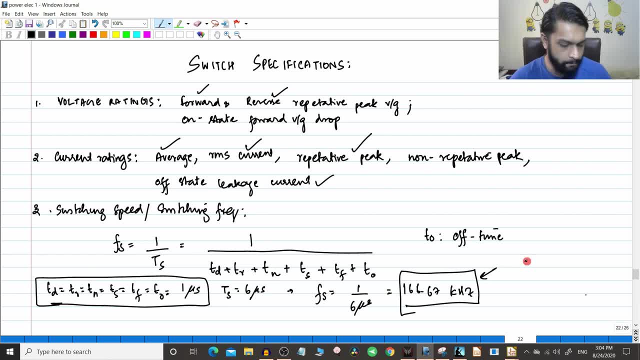 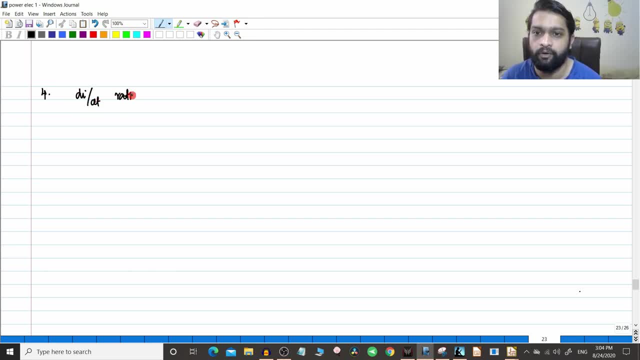 okay, so this is another specification that the manufacturer gives to the manufacturer will give then the next thing is called the di by dt rating. di by dt rating now based on the loads which are connected to the system. sometimes you might have huge di by dt, right you might have. 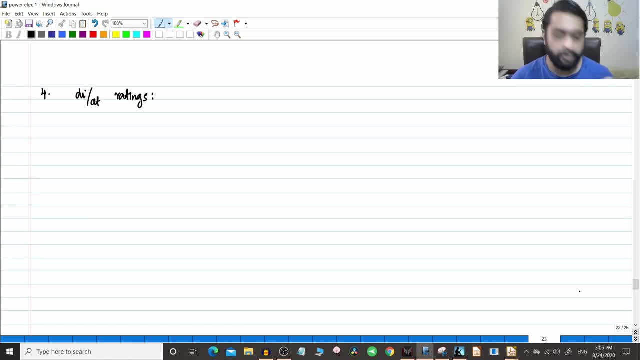 the device might encounter high di by dt. so in that case, uh, what happens is that when there is, like, when there is sudden increase in current, the current which it might not be able to spread throughout the device, right so there might be localized hot spots, localized di by dt, and this localized hot spot will actually cause damage to the device, unless 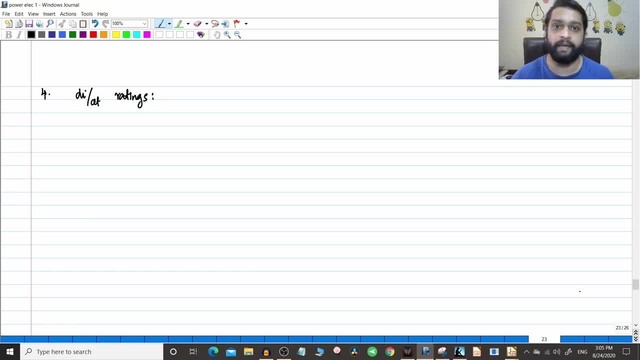 the heat is properly dissipated throughout the device, it might cause damage. okay, so the idea is that when the current increases rapidly, when the current, when the current increases, increases rapidly, okay, when the current increases rapidly, uh, the current, the current might concentrate. current might concentrate, so you can also take down: current might concentrate at localized areas. 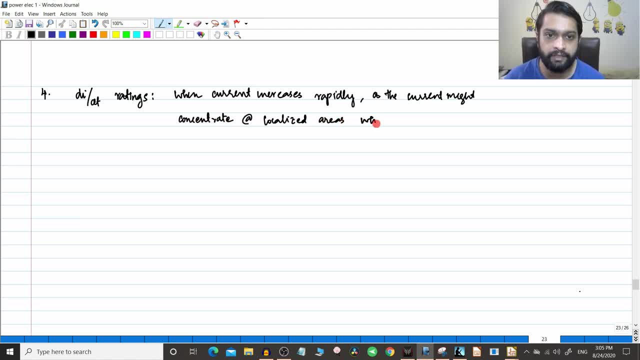 at localized areas, which creates hot spots, which creates hot spots, which creates hot spots, and this can damage the device, and this can damage the device due to overheating damage the device. so, to prevent this, there is a specific circuit which we will, of course, deal, uh see, in detail. 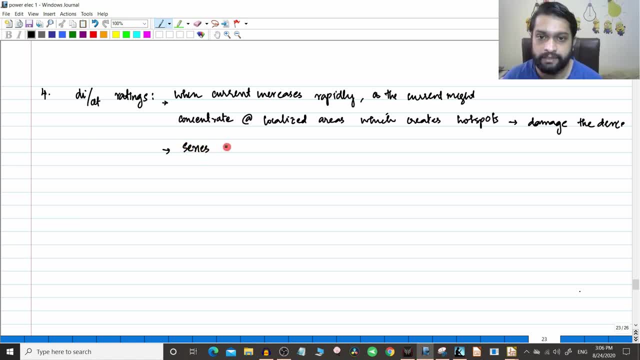 which is called the c series snubber. So if they ask in some objective question, even without studying that, you can understand that series snubbers are used to limit the effects of di by dt, So snubber is used to limit the effects of di by dt. Of course we will be seeing all these things. 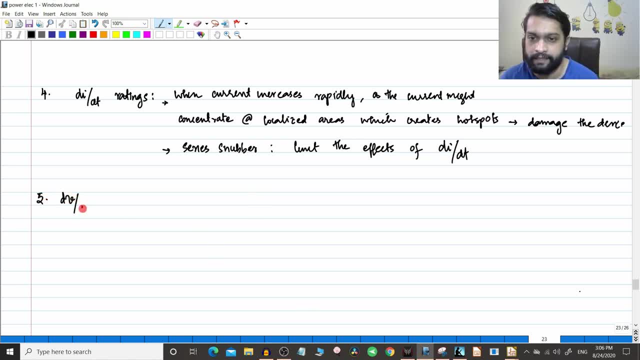 in the future videos. And next is the dv by dt rating. Now you know that any of the semiconductors. if you have learned a little bit of analog electronic, you are having something called the junction capacitance. You are having something which is called the junction capacitance. 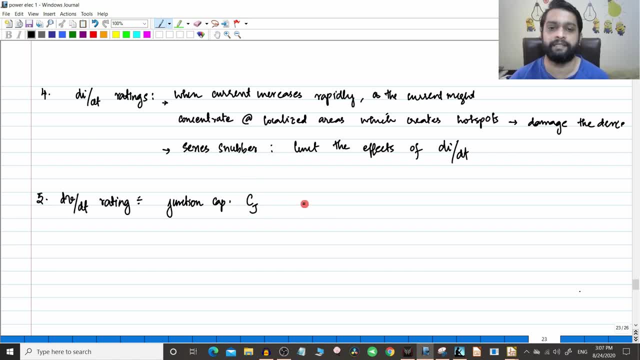 which is called Cj. Now, because of this junction capacitance, especially during starting conditions, you can have a current which is called Cj dv by dt. The value of that current is Cj dv by dt. Now, if there is sudden voltage surges, if dv by dt is very high, 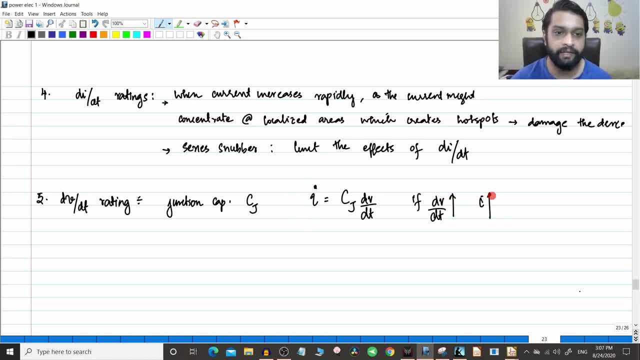 this current is going to be very high. So if there is sudden voltage surges, this current will become very high. This junction current will be very, very high And this can also damage the device. This can also damage the device. Therefore, the manufacturers 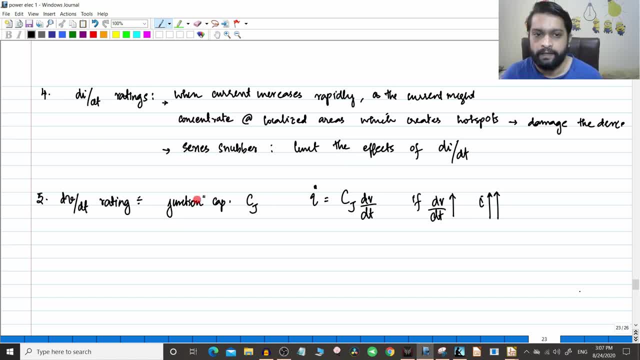 will give you a limit of dv by dt rating also. So this is also another problem here. So to prevent, limit the effects of dv by dt, you use something which is called a shunt snubber. So di by dt rating is, or the effects of di by dt is limited by series snubber and 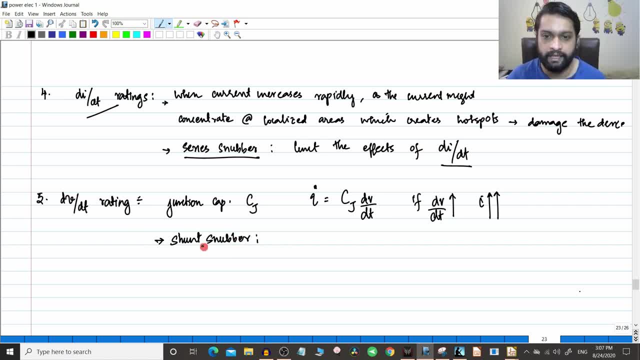 effects of dv by dt rating is limited by the shunt snubber Limit. the effects of dv by dt rating: dv by dt, not dv by dt, dv by dt in general. Now the next point is the switching loss. switching losses Now in the previous videos we have already seen whenever there is a switching. 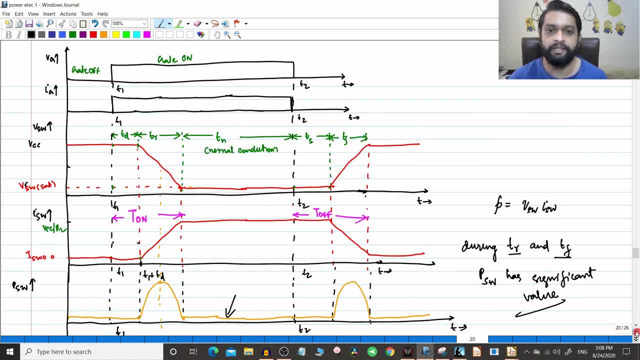 which is happening. right. it can be in the turnoff condition or in the turnoff condition See. now it is turning on at this point. So this is the gate pulse given. So once the gate pulse is given, you see that there is a peak. 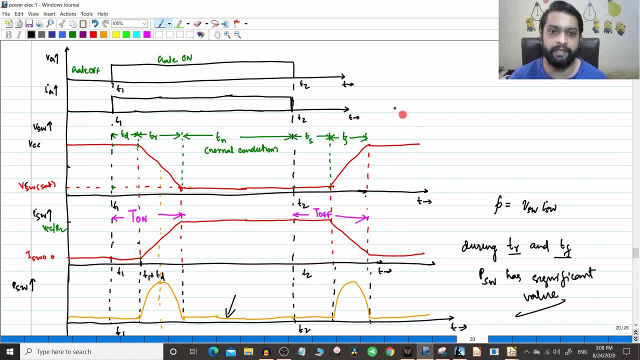 here: right, there is a peak here. Similarly, when it is turning off, there is a peak here. Now, after some time, for example, you are giving another gate pulse, there will be another peak like this in power. And when you turn off that, there will be another peak like: 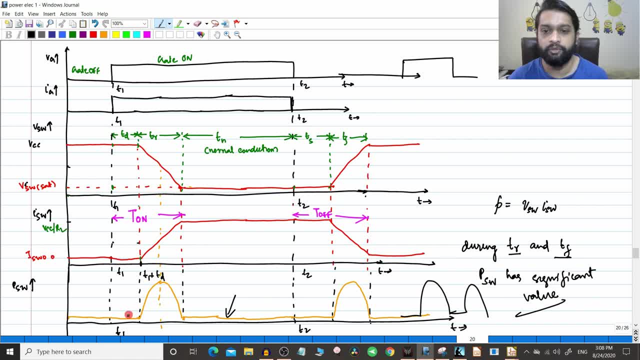 this. So, depending upon the frequency of operation, you will have continuous peaks like this And I have told you this: switching losses is much high, especially in the turnoff, especially in high frequency circuits, as compared to the on-state conduction losses as well as the overall gate requirement. 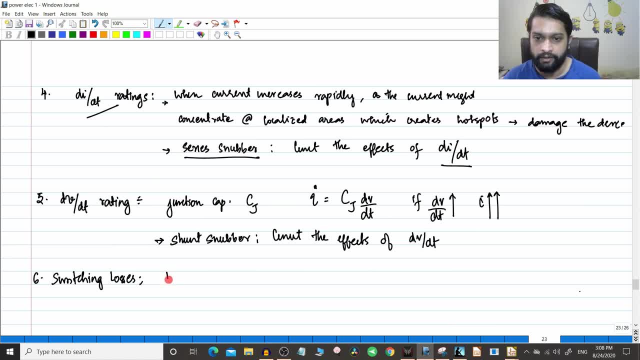 So we have already seen that the switching losses or the P switching, is very much higher as compared to, as compared to the on-state power loss and the gate drive power losses, So especially in high frequency circuits, especially in high frequency circuits. So 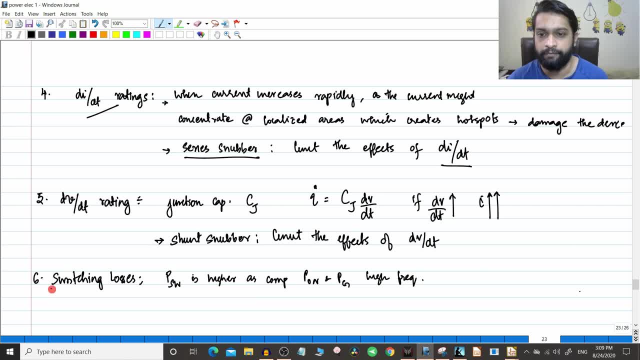 this factor is also considered. So look at the temperature, what she jumped here. So something going to be very important, okay, so the manufacturer will also give you an idea of the switching losses associated with the circuit. okay, why this is important? because this is a significant 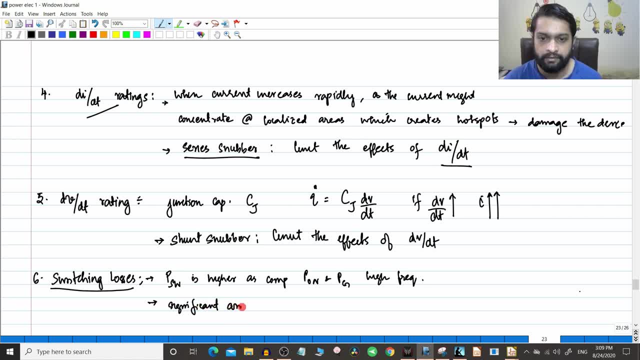 component. it is a significant component of the overall power loss, overall power loss of the device, overall power loss of the device. because you see, there might be multiple devices like this, not only scr, there might be other devices. so when i manufacture of an overall device which might contain many semiconductors, many power electronic circuits must have an 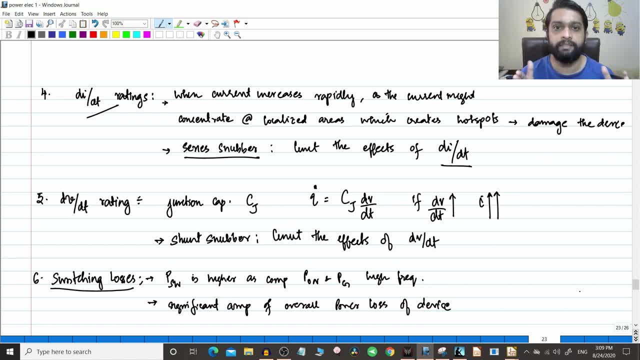 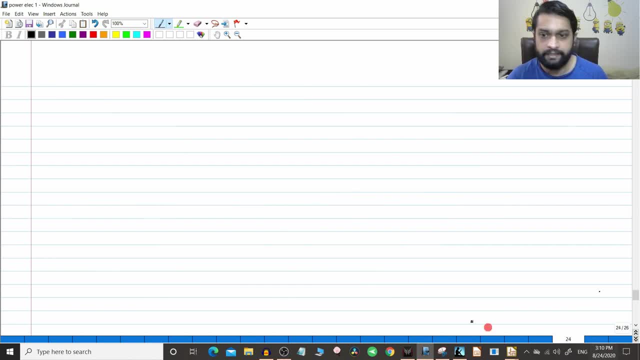 overall loss, how much loss this is going to cause in my overall system. so he should have an idea of the switching loss. so these are also usually given in the data sheets. next is called something which is called the safe operating area. safe operating area. okay, now if you draw a simple vi characteristics: 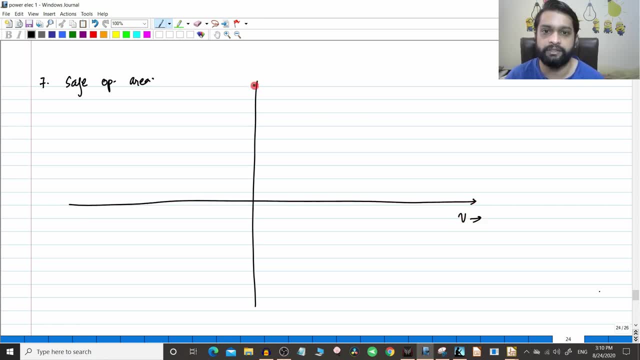 okay, depends on the case. okay, so this is the voltage across the device and this is the current. okay, we can call. is WN VSW, voltage across, is its current across the switch. now you should have always limits on the voltage and current. why you should have what limits on voltage and current? because 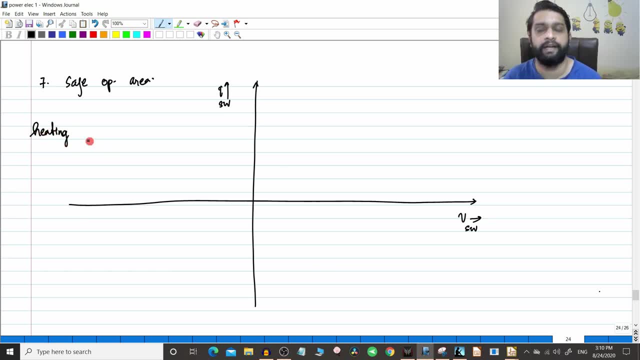 see the heating loss, the heating on the device. heating on the device directly proportional to the power loss. right, because what is heat energy? energy is nothing but power into time, so heating is actually to the power loss associated. Now, what is power loss? The product of voltage and current The 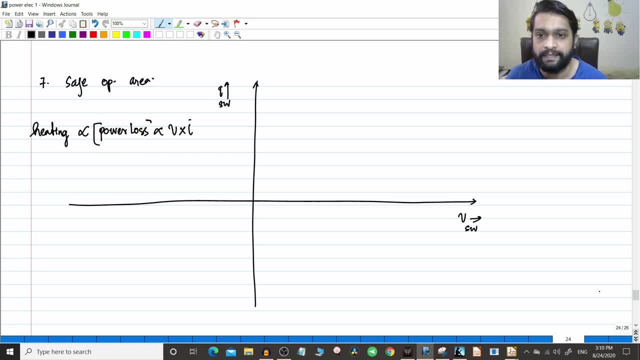 power loss should be voltage and current. Therefore, when you are setting a maximum value of the power loss, you should have a maximum value of the power loss of the system, beyond which the machine will get damp or the device will get damp. Therefore, you should set a maximum for this. 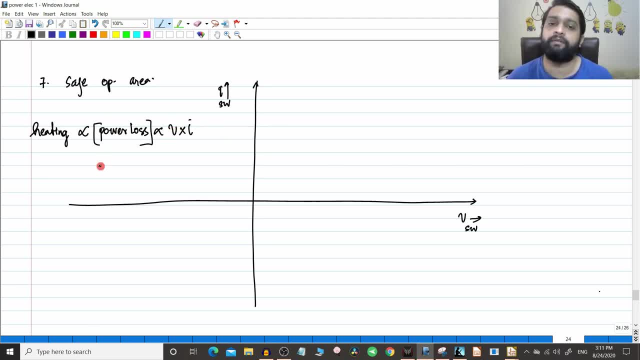 power loss. So, and this maximum power loss should be constant value, right, It should be constant, it should not be keeping on varying. The maximum power loss will be a constant value, okay, So the maximum power loss, the power loss maximum, should be a constant value. How it will be? 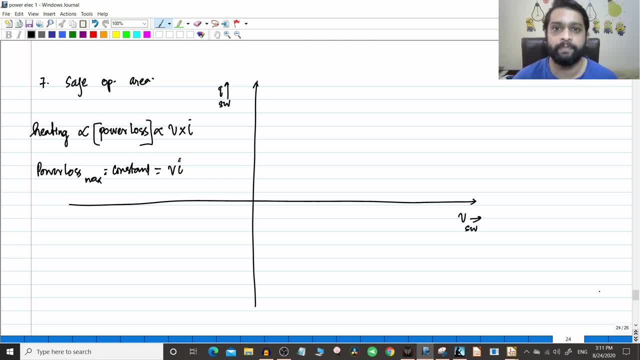 constant. It will be constant if Vi is equal to a constant value. If Vi is a constant value, what it means is that the voltage is a very high value. the voltage is a very high value, then current should be a very low value, okay. So what it means is that the device characteristic 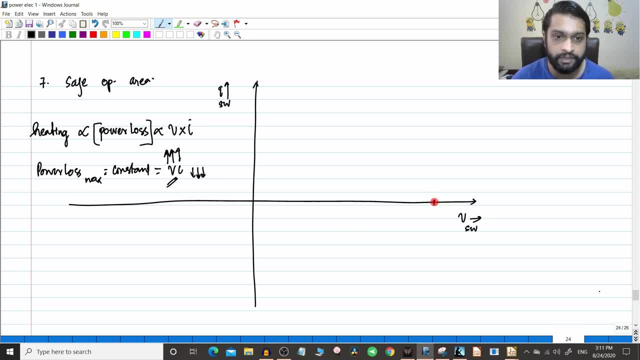 should be in such a way that when voltage applied across the switch is very high, is very high, that it, for example, this is V max. okay, That time the current should be very low. The current should be some I minimum. okay, Then only you will have this constant. 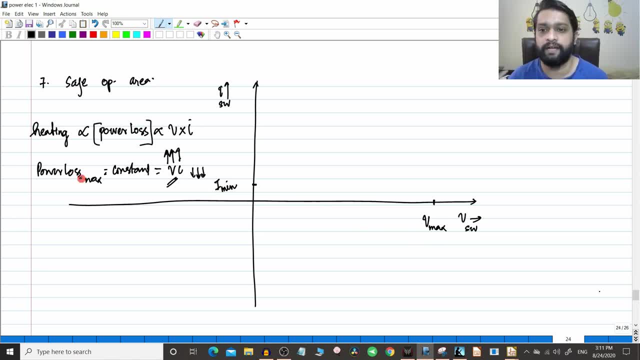 criteria. okay, So when voltage is very high, the current will be very low, so that this power loss is maintained constant. So, for example, if you take these two points, this will be the operating point of the device. right, This will be the operating point of the device, okay, So 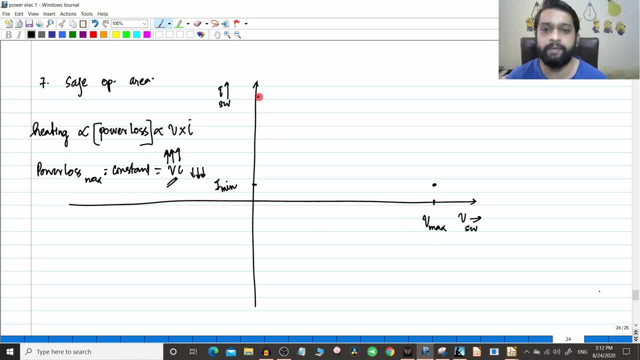 it should work in this particular. this is the maximum operating area. Now, for example, the current is some I max. okay, So to make the voltage, the power loss, constant. if the current is very high, the voltage should be very low. So voltage will be some V minimum. 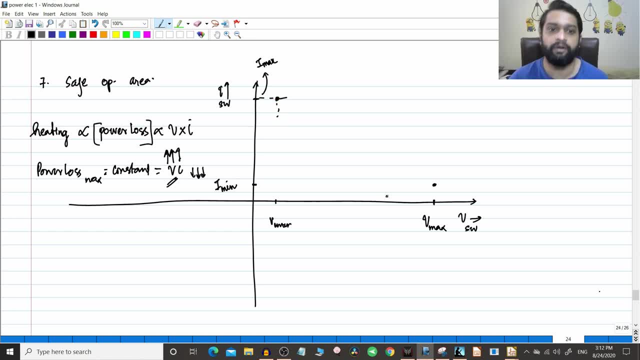 right, So this will be the working point. right, So this will be the operating point. okay, So for example, in this area here the voltage is 0. So when you are increasing, keep on increasing the value of voltage from 0 to this V max, the current has to drop like this: 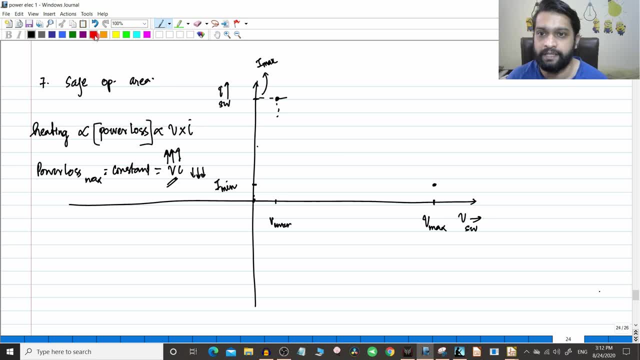 the current has to drop like this. okay, So if the current is very high, the voltage should be 0.. So if the current is very high, the voltage should be 0.. So if the current is very high, the 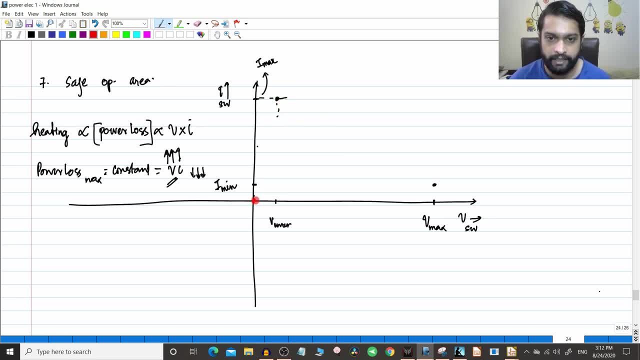 characteristic for the safe operating area will look something like this: So when you are increasing the voltage from 0,, 1,, 2,, 3,, 4,, 5,, 6,, 7, like that, so the current value should decrease. 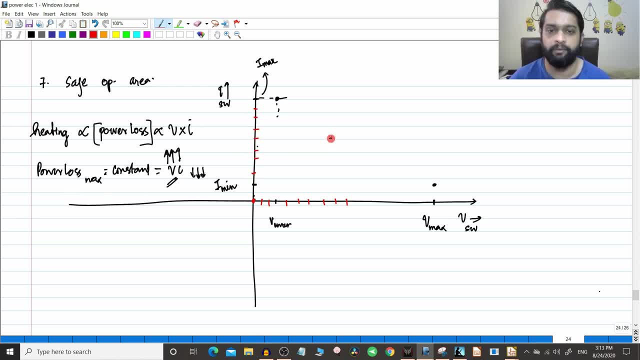 then only this maximum power loss will be constant. okay, I hope I am clear. So the characteristics will look something like this. So it will be a graph which is looking like this: okay, It will be decreasing. okay, So this is the operating area, So you can have the same. 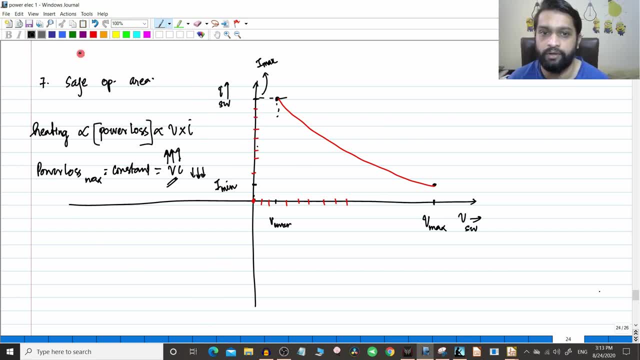 operating area in all four. Okay, So this I have drawn only for the first quadrant. So if you have some mark, some areas like this, So this is one area, this is another area, this is another area, all four quadrants. 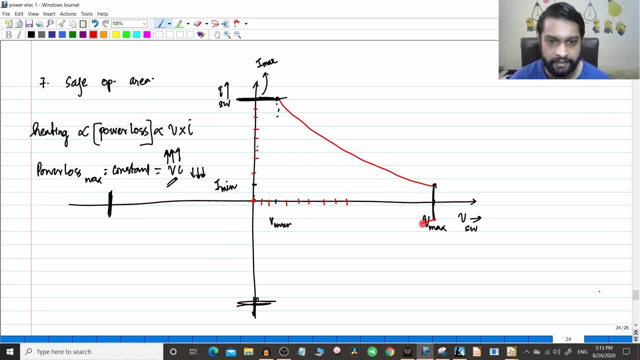 we can mark this safe operating point. So everywhere that relation will hold good. So the safe operating area will be something like this: So inside this quadrant you are having safe operating area of the device. We have seen this in synchronous generators also. If you 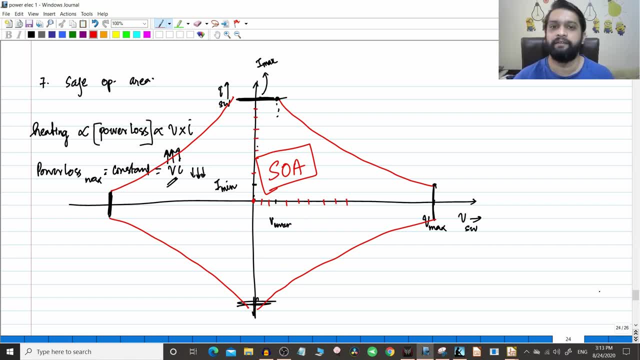 remember when we were drawing safe operating area of synchronous generator. we have drawn all these things. So beyond this, this is not safe operating area. If your machine is going beyond this, if device is going beyond this characteristic, it is not safe and here it will get damaged. This portion you should not. 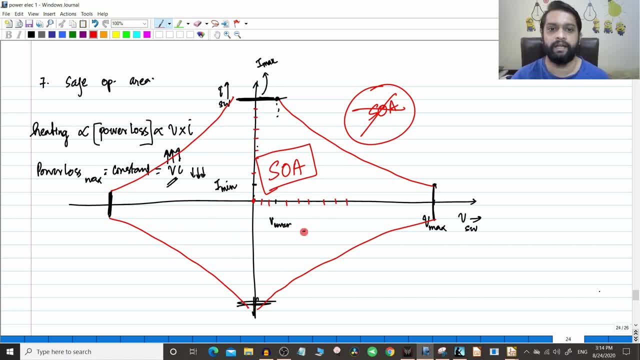 work. You should always try to work your machine inside this particular area, and this is the line. This line here shows you constant P max. You can call it as constant P max. This is also constant P max. Yeah, this line is showing constant P max. 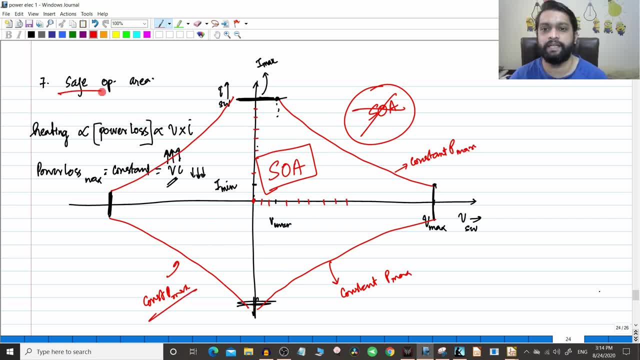 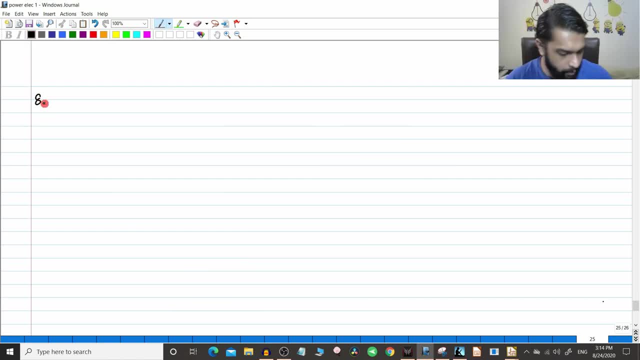 This is also constant P max. Okay, So I hope I am clear, so you always have a safe operating area of the device. Now next is the next point is called i square t for fusing. This is also usually given in. 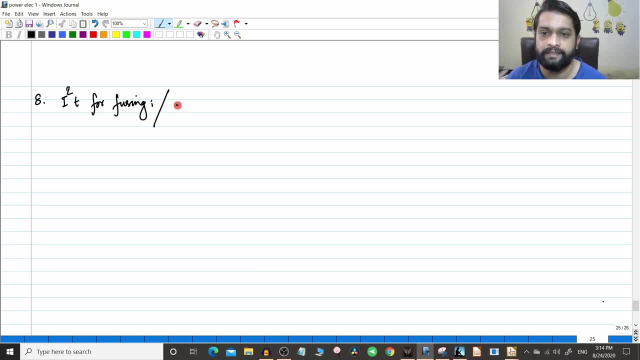 the data sheets. Now this i square t is also called as the melting integral. melting integral, Okay Okay, also called as melting. Now this is actually used in the power supply part. So this is actually used for this device rating- Usually all semiconductor manufacturers, that is. 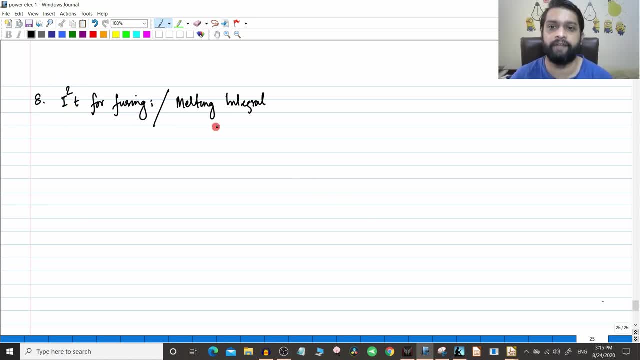 especially SCR MOSFETs, IGBTs. they will give this I square T value. This is called the melting integral. This is used for fusing. So that is another concept altogether- People who are manufacturing these type of power supply. they will need this value to determine what should. 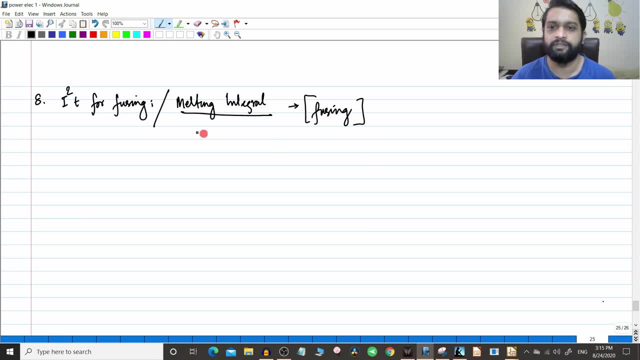 be the fuse which is used in this power electronic circuit. So just for the time being, understand this, I square T is also given, which is also called as the melting integral, and it is used to give the fusing of the circuit. Now, that itself is a big calculation. It is not. 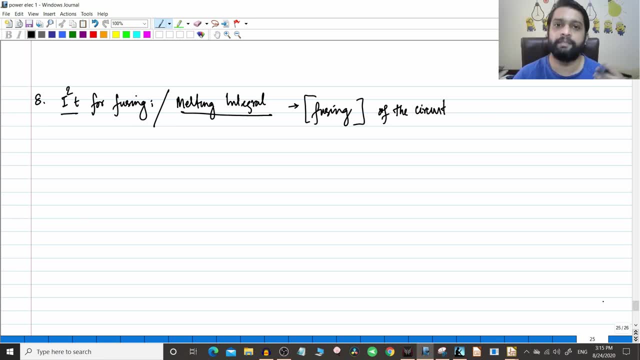 only this, I square T, which is used for fusing calculations. There is, depending upon the voltage waveform applied in the power circuit, the temperatures. there are so many factors which you take into consideration before deciding on a fusing, So this is a big calculation. 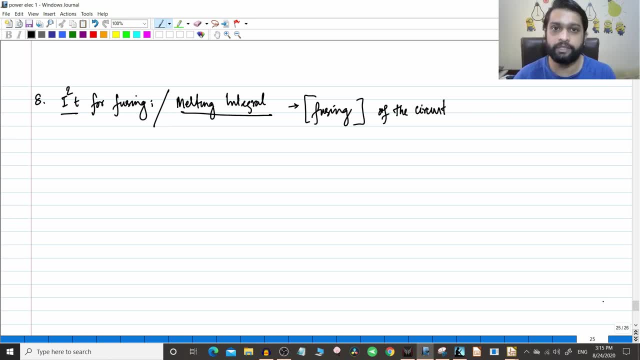 The time which is required for the fusing to happen. So there are a lot of conditions. So you cannot just tell this. I square T is the only quantity which is used for fusing. Other than that, there is a lot of conditions. But just for the time being, remember that I square T is also 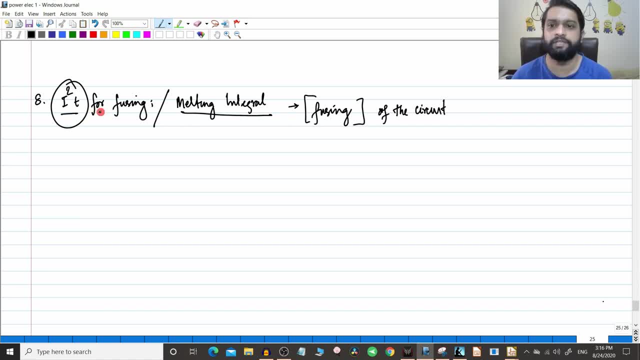 given as a rating of the semiconductor or the SCR or the switch for the fusing conditions. Now they will also give you information about the temperature limits of the device. So they will give you the temperatures like this: Usually if you take a 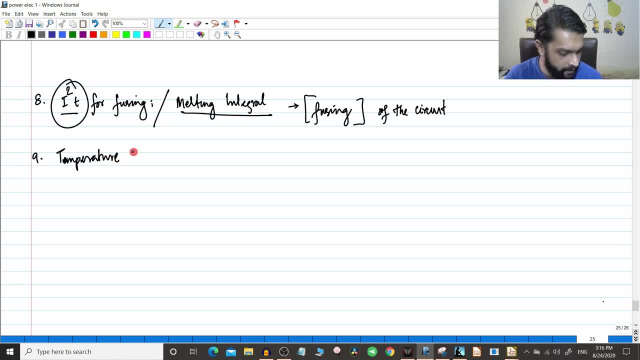 data. you will get a data of the temperature limits of the device. So you will get a data of the temperature limits of the device. So you will get a data sheet. you will find something like this: In case of temperatures, they will give you a junction and case: temperature Junction and case. 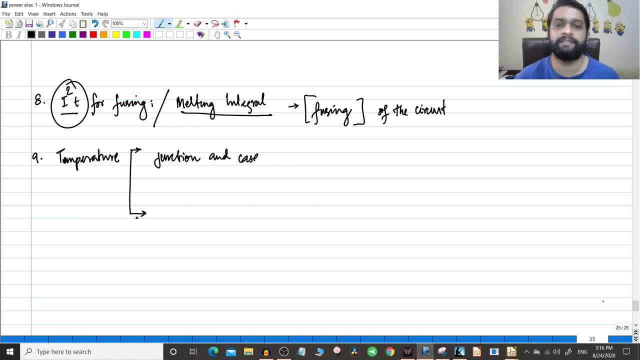 temperature. That is the allowed maximum which they have calculated before the device might fail. So that is usually 150 degrees to 200 degrees C. This is the allowed, And other than that they will give something else which is called the storage temperature. That is the ideal conditions. 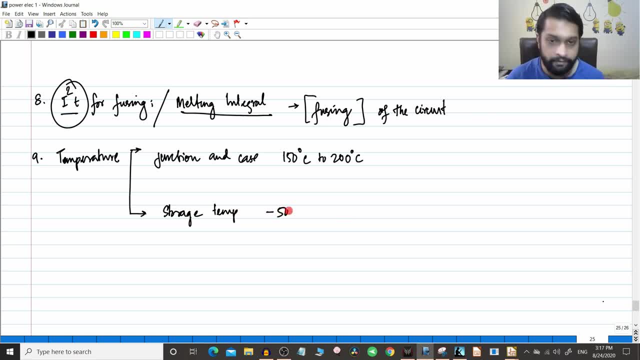 in which you can store the data. So that is the allowed maximum which they have calculated before the semiconductor. So that is usually minus 50 degrees C to 175 degrees C. These are all arbitrary values, not arbitrary value, usual values which are found in a lot of manufacturers. If you take 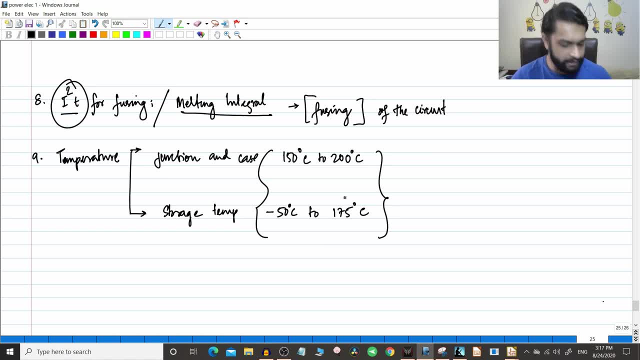 a specific manufacturer, they will give what is for that particular device. Now, another important thing is the gate drive requirements. I forgot to write that Gate drive requirements. Now I already told you the gate circuit which is actually driving, the actual mechanism of when. 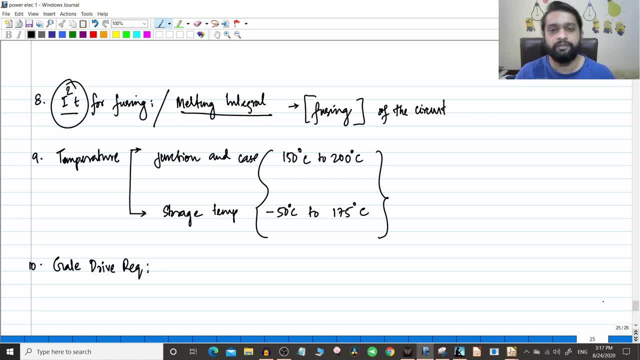 the switch should turn off When the switch should turn on. it is an integral part, So that is also very important. Sometimes in certain type of devices you will need a continuous gate pulse, But in some devices you might only give a small gate pulse. It will turn on. Then you can stop the gate pulse. But 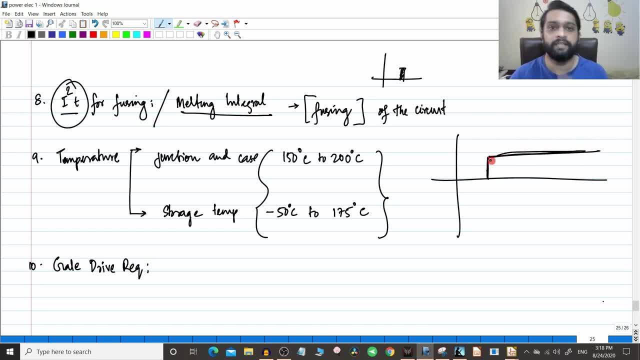 for some devices. there are devices where you need a continuous gate pulse like this for it to work for a particular operation. In some cases you just need a small pulse. So in those type of circuits also you are having gate pulse, So in some cases you just need a small gate pulse. So 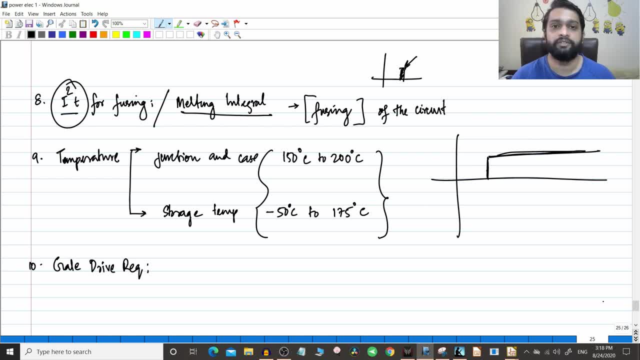 in some cases you just need a small gate pulse. So in those type of circuits also you are having a significant gate drive loss. So the gate circuit is a separate circuit that also will have some power loss. So that is gate drive requirement, which is also very important. Now the next point is called: 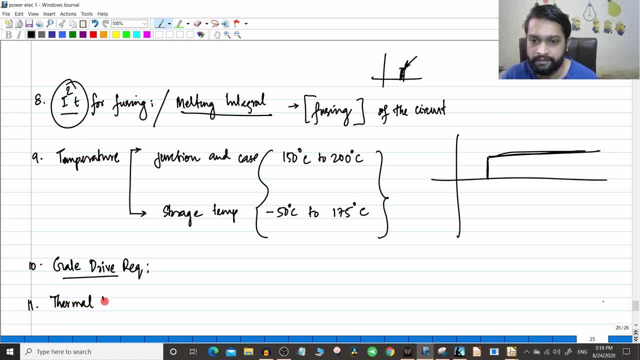 the thermal resistance. That also they will give in the data sheet thermal resistance. So in thermal resistance there are multiple data they will give. One is called junction to case. Then you are having case to sink, then you are having sink to ambient. 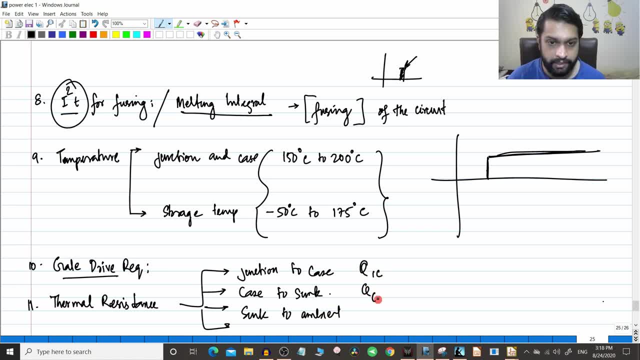 So this is Qic, Qcs, Qsa, Qjc, Junction to case means from the actual semiconductor, actually the junctions of the semiconductor, to the case of the thyristor or any device or the case of the switch. So that is this thermal resistance. 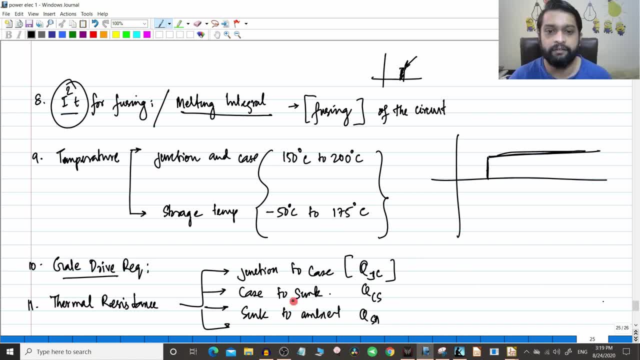 These are also used by designers etc to do various calculations. Then from the case to sink. Now, usually if you see a semiconductor, you have the semiconductor case like this and you will have some leads like this and over this you will have a heat sink. 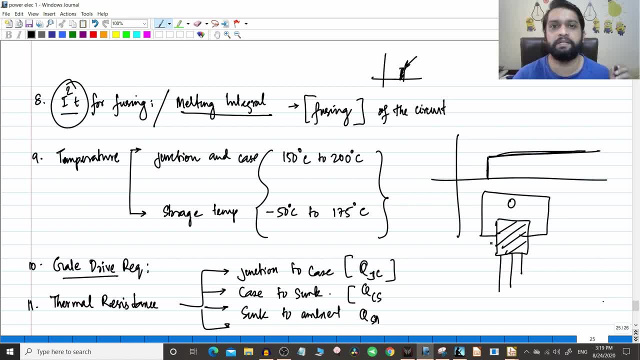 Because this semiconductor, if you just keep like this, it will burn off instantaneously because that much amount of heat will be produced. So you always you need a heat sink like this, which is usually provided by the manufacturer, but in for just In case of protection, usually designers will add heat sinks so that proper heat dissipation happens. So the basic idea is that because some devices are working at very high frequencies, a huge amount of switching loss will be avoided. So as soon as possible that heat loss should be removed from this particular device. 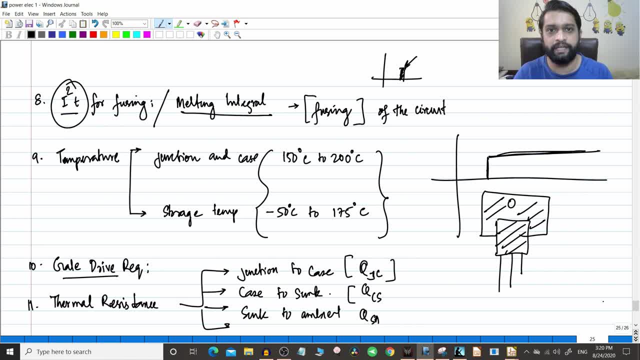 So that is a basic idea. So as soon as the heat is produced, it should not be allowed to stay there, It should be removed, It should be taken to the ambient. So therefore you are having junction to case, thermal resistance, case to sink, which is 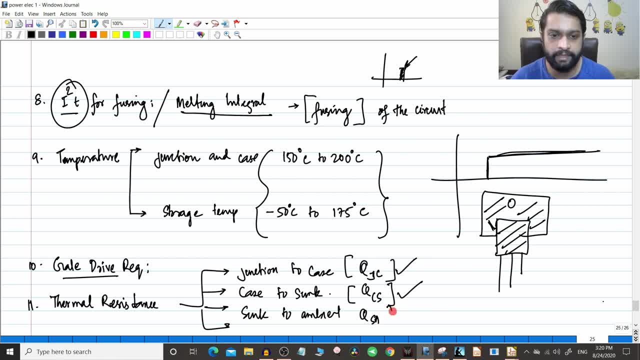 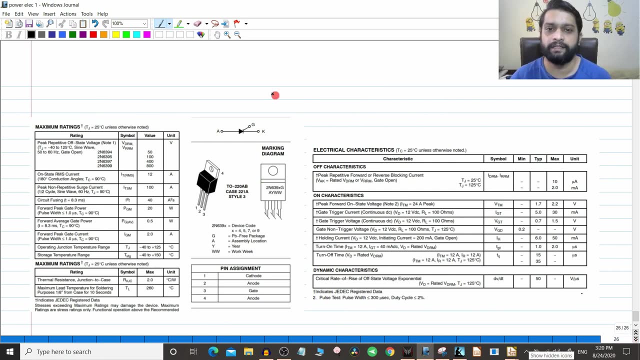 this is case. So the heat sink, in between this one thermal impedance will be there, and then from the sink to ambient. These are also other conditions which are given here. Now let us see manufacturer data sheet of a switch. So this is a simple data sheet which I have taken. this is from on semiconductors of their 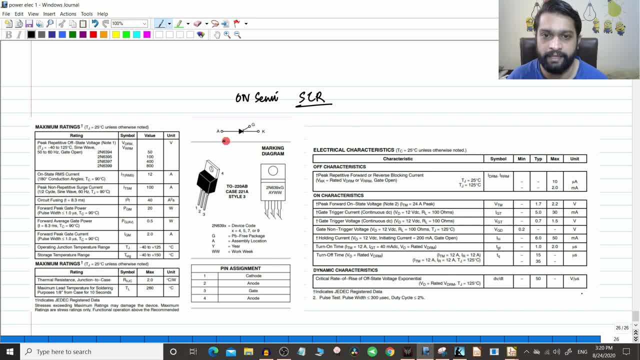 silicon control rectifiers, SCRs, So you can see the symbol here- anode, cathode and the gate circuit. So you see, here you are having peak repetitive off state voltage. So we saw that already, Peak repetitive off state. Now they are having two or three models here. 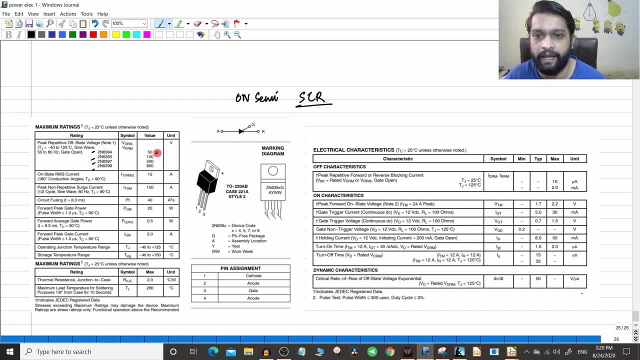 So one, two, three, four models they are having. So, depending upon the model, they are having 550, 100, 400 and 80. So this is the peak voltage. Remember this is not the RMS. well, this is the peak voltage. 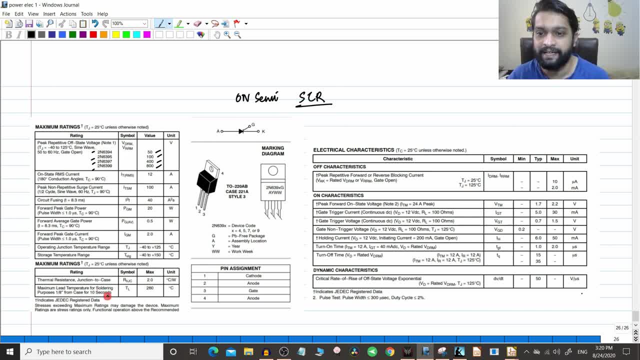 So that is called as VDRM and VRM. Now why I have stated this data sheet? because they have given the explanation of what individual symbols are, So this is a very good data sheet. Then you are having see on state RMS current. 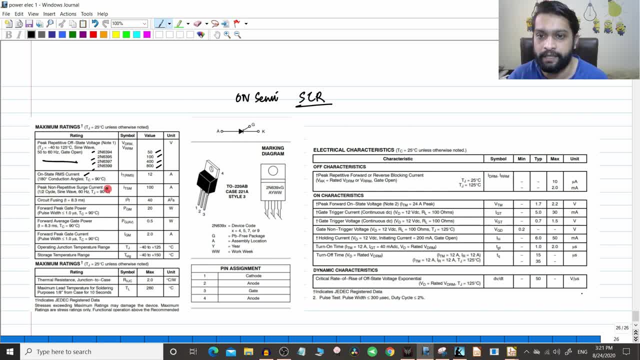 We have already seen that one. The RMS current is also. they will give it then peak, non repetitive stirs current. So I told you these are surge current, So not all currents are repetitive. So repetitive currents will be the part of the normal operation of the circuit. 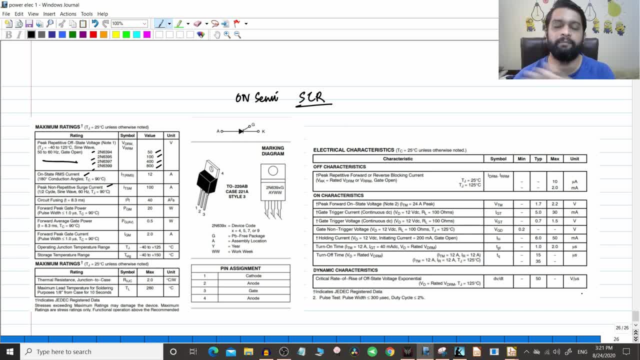 That is why they are keep on repeating. but this surge currents is not repetitive. It might be in the starting position or the ending position or suddenly some non linearity is coming into the system, like lightning strike or something like that, That is going to introduce this non repetitive stir surge current. 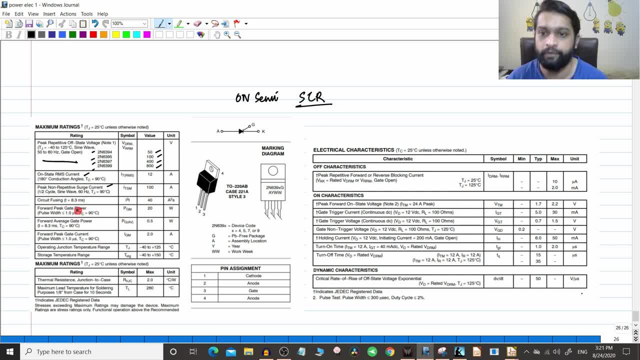 So for that also they have given a rating here. Then they have given: see: circuit fusing: i square t. you can see here i square t. i think it's a little bit small, but i hope you are going to understand. so this is i square t, so that also they have given then see: 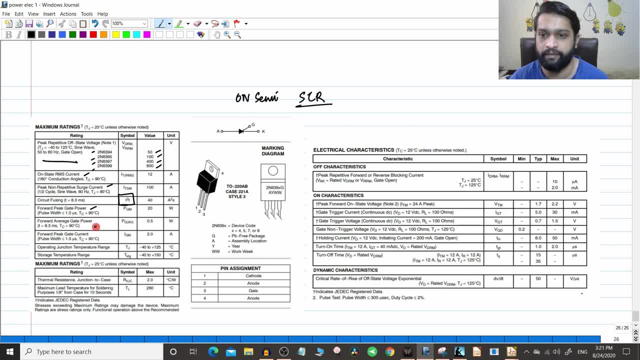 for gate power requirements, forward peak gate power- that also they have given average gate power. they have given average peak gate current. they have given. then see operating junction temperature, see this: they have given operating junction temperature range and they have given storage temperature range. so these are all things that they give. and then you see thermal. 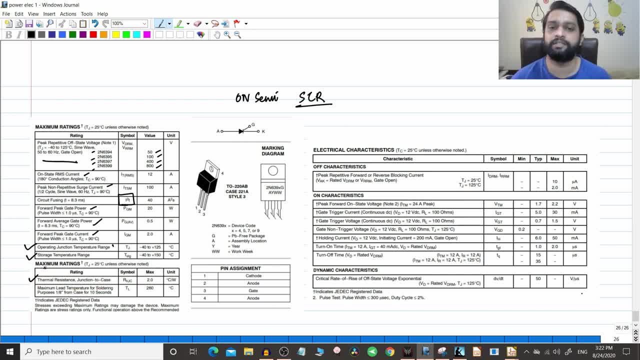 resistance junction to case. they have given thermal resistance junction to case. okay, because this is the actual device that they have given for the junction to the case. okay, and other than that, let us see what all they have given. see, they have given peak, repetitive forward or reverse. 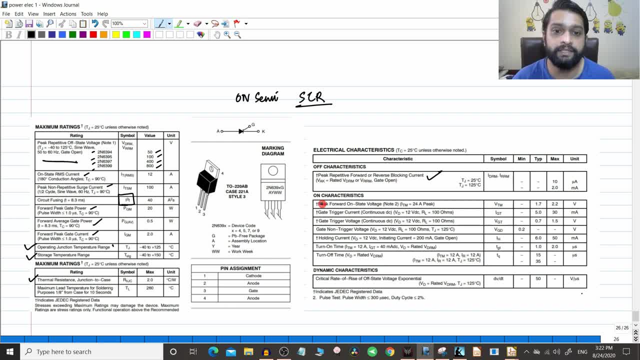 blocking current. also they have given that. they have given then for on scare statistics. so they see they have given forward on state voltage, drive on right forward on. so you can see the values are typically 1.7 volts. okay, so ideally it should be zero. but see now gate trigger current. they have given gate trigger voltage and holding current. 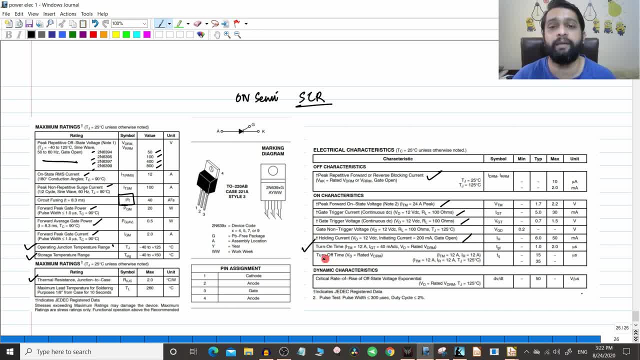 which will come in the future video. then you see the turn on time they have given. turn on time is delay time plus rise state and turn off time also they have given. so you can see all these values. you can just google um scr space data sheet and mostly you will get this data sheet in the first. 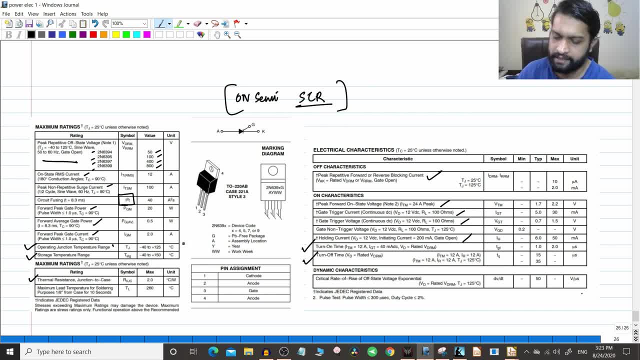 result itself. so this is the basic idea. another thing is that see, teaching you people. uh, about the devices, device characteristics, there is a certain limit to it. now, after your college, when you go into a job, no, they might give you a small training or something, but after that, for the new, new, new challenges that you are going to face in, 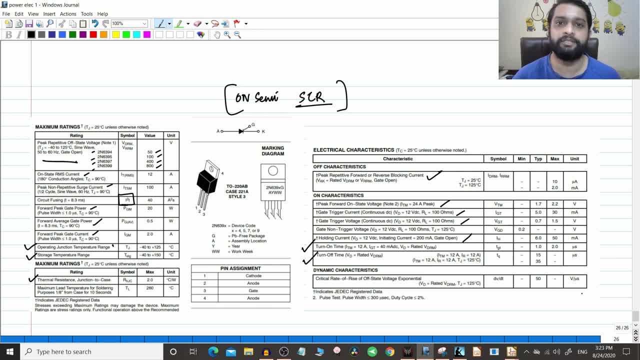 your life, in your professional life, nobody is going to come and teach you. that is why i always urge people to learn subject on their own. okay, even before watching all these videos, you should try and attempt to learn the on your own, because that is very important, because in your life, in the future, nobody is going to come. 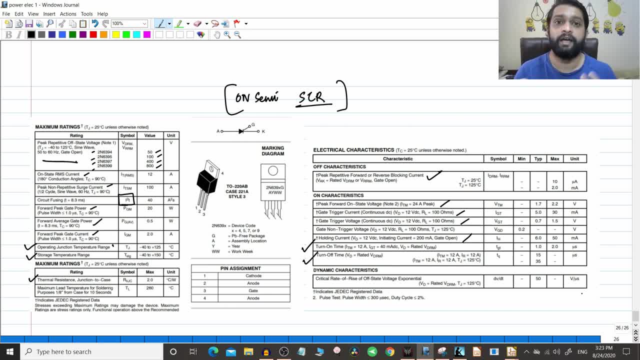 and teach you everything, so you might have to go through data sheets. you might have to learn a lot of things on your own. for for everything, you won't have youtube videos. see for a btech, for an engineering course like this. you might have hundreds of videos, but when you are going, 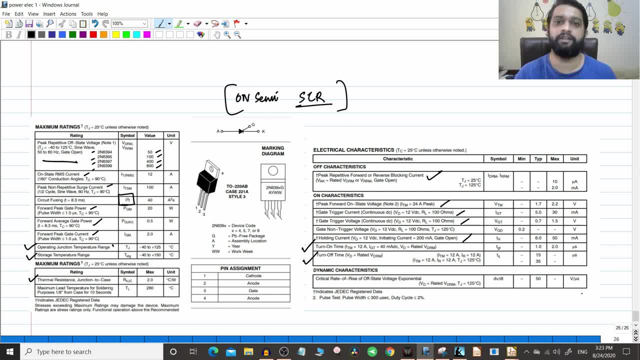 to talk about a professional career, professional technological, technology based career. see, not everything is given for free. for example, a particular manufacturer has a particular software and all those things, but they might ask you money if you want to learn from them. okay, not everything is given for free. so if you can learn on your own, that is the best way you 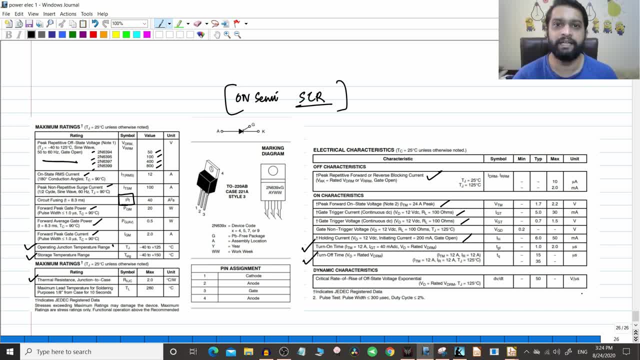 don't have to pay them any money because ultimately they will be giving all the data sheets. they will give you all the information. so the trick is to learn. go through these data sheets, go through, go through the documents and learn a lot of technologies on your own also. so unless you 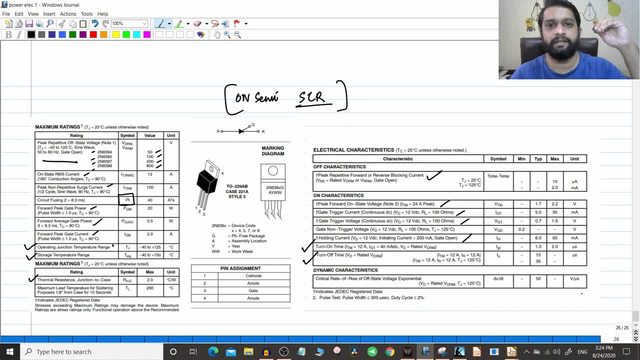 develop that habit, getting to a point that is, you can do with all these videos, but after that you should put your own efforts to understand things. so that is why that habit you have to bring in your life now. okay, so i think that is enough for today. in the next video we will be just going through various 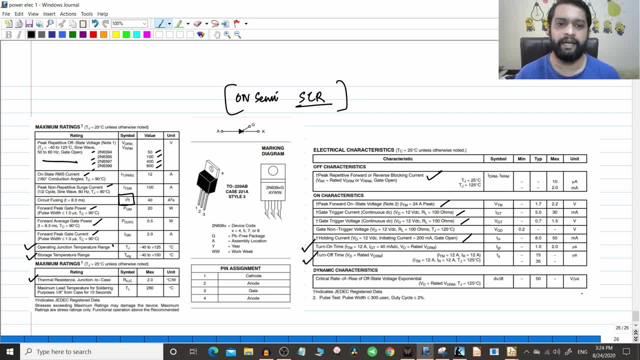 types of power semiconductor devices. mostly it will be a theoretical time based explanations. we'll just see what all type of power semiconductors are available in the market. okay, so till i see you in the next video is me, varun. have a great day, thank you. now that the video is over, please stay with me for 30 more seconds.